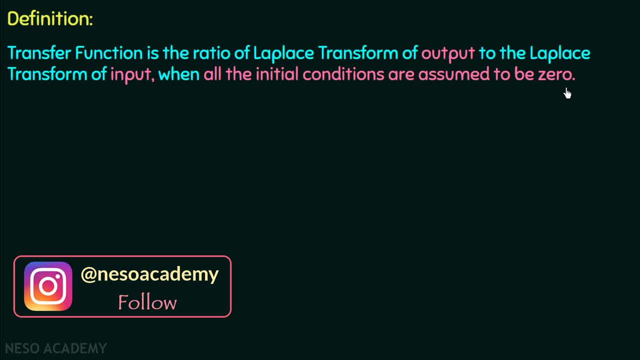 This point- all the initial conditions are assumed to be zero- is a very, very important point. We cannot define the transfer function without assuming the initial conditions to be zero, And it is because we define the transfer function for LTI system and in case of LTI, 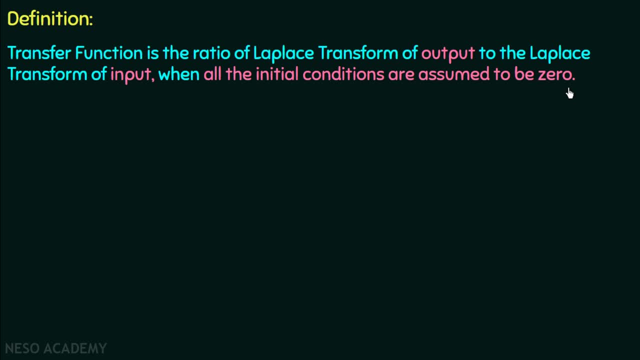 systems, all the initial conditions are assumed to be zero. We have discussed the reason in the previous lecture. If the initial conditions are not zero, then the system will not be a linear system and hence the system will not be LTI. That's why, to define the transfer function, all the initial conditions are assumed to 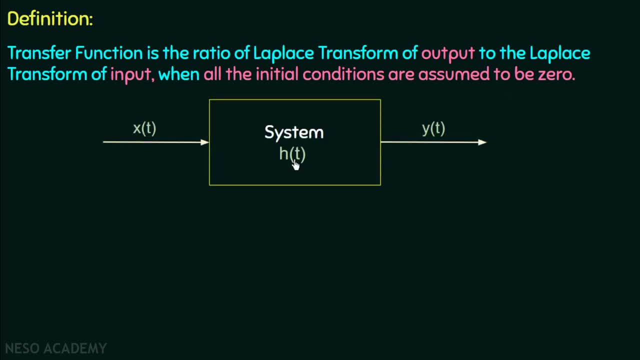 be zero. Now suppose we are having a system which is, of course, an LTI system and its impulse response is h. We are giving an input x to this system and its response is y. Now we all know that y is equal to the convolution of these two functions, So we can write y. 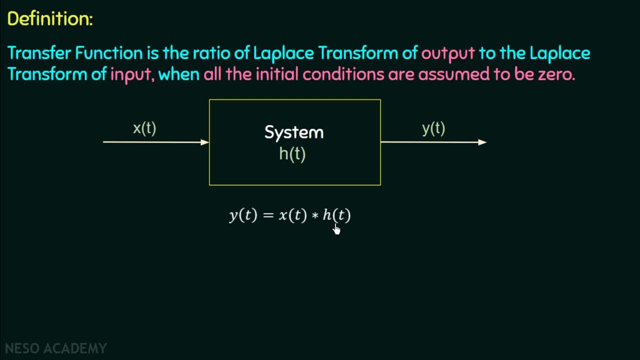 is equal to x convolution with h. And from the convolution property we know that the convolution in time domain is the multiplication in frequency domain. So by convolution property we can write: y is equal to x multiplied with h, where y is the Laplace transform of y. 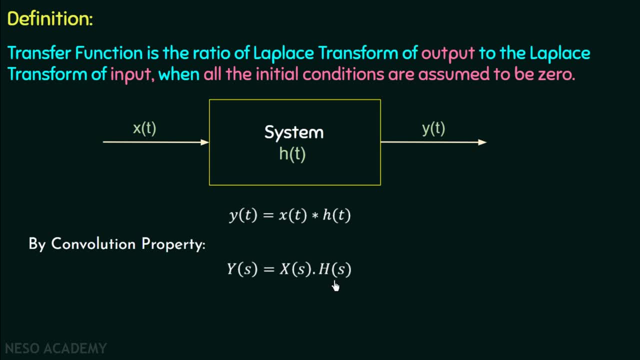 x is the Laplace transform of x and h is the Laplace transform of h. Now, from this equation, if I take the ratio of y to x, then we will have: h is equal to y over x and this is the transfer function of this system. 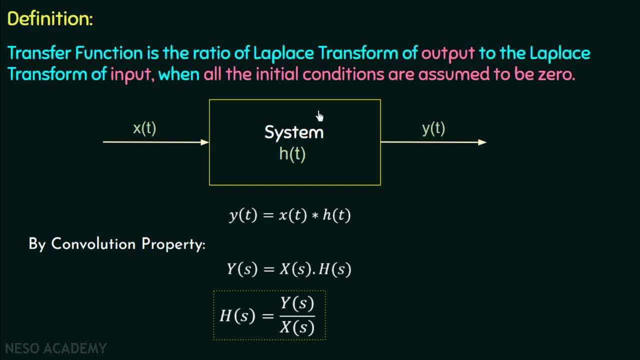 Now here we have defined the transfer function for this system and we know this system is an LTI system. So by default, in this case the initial conditions are equal to 0. But if we define the transfer function for an arbitrary system, then in that case the 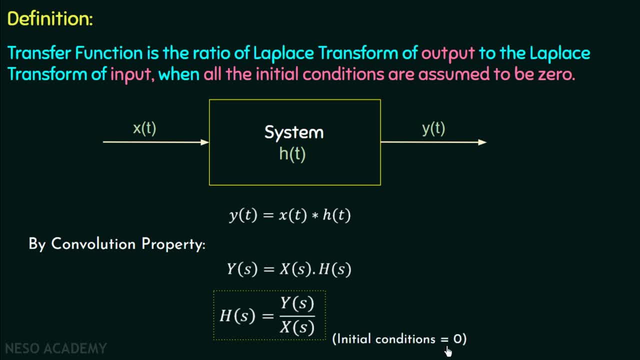 initial conditions must be equal to 0. And to understand this in a better manner, we will take one example. We can also notice that h is the Laplace transform of h, So we can say that the transfer function for any LTI system is the Laplace transform of the impulse response of that. 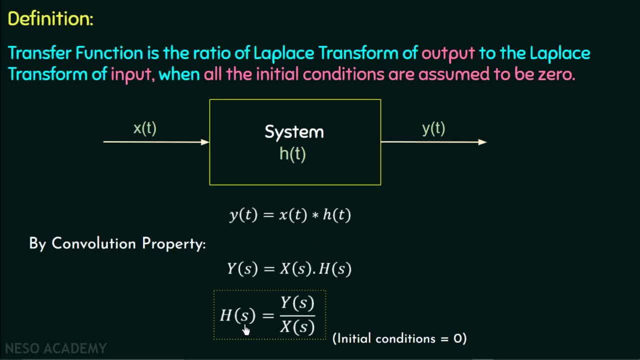 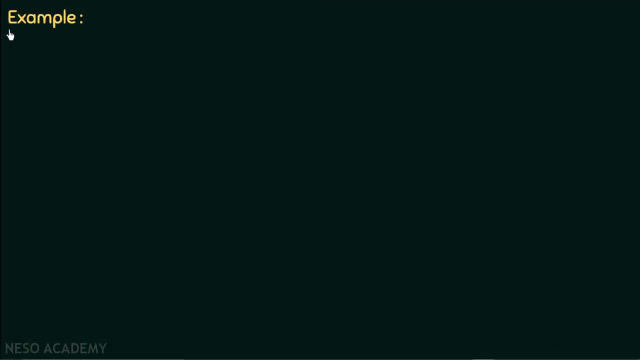 LTI system. Suppose we are given the transfer function of an LTI system and we are asked to calculate the impulse response. then we can calculate it easily by taking the inverse Laplace transform of h. We are going to solve many such questions in the upcoming lectures. 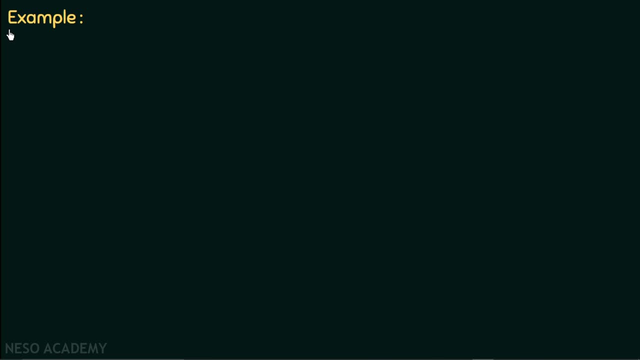 So now we are done with the introduction of transfer function. Let's take one example to understand it in a better manner. And the example is given as: find the transfer function of the system given by d square yt over dt square plus 3, multiplied d yt over dt plus. 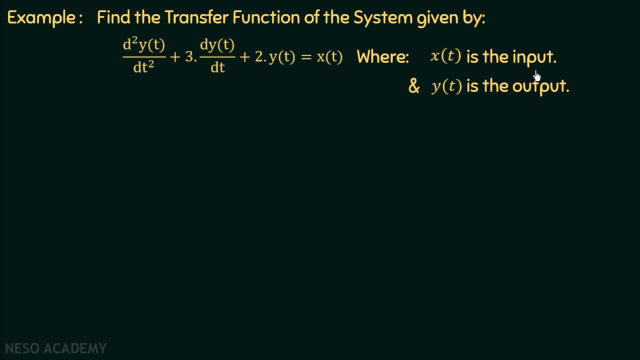 yt is equal to xt, where xt is the input and yt is the output. So we are given a system which is defined by this differential equation, where xt is the input to that system and yt is the output, And we need to calculate the transfer function. 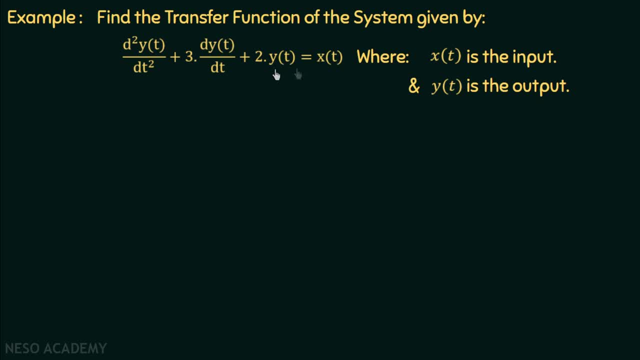 And we know the transfer function is the Laplace transform of output to the Laplace transform of input. Now, moving on to the solution, if we take the Laplace transform on both the sides, then the Laplace transform is equal to xt, where xt is the input and yt is the output. And we 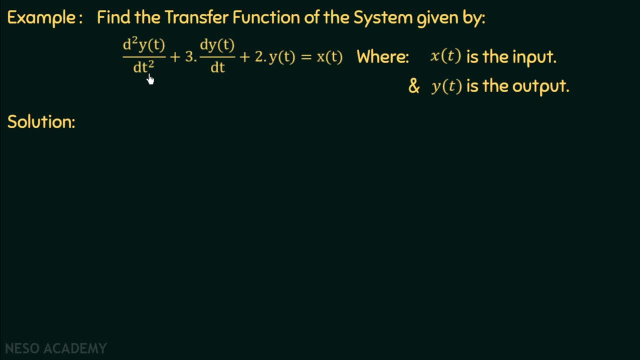 know that the Laplace transform of d square yt over dt square by time differentiation property is given as s square ys minus y0 minus minus y dash 0 minus. Similarly, the Laplace transform of d yt over dt will be s ys minus y of 0 minus, And it is multiplied with 3, so by: 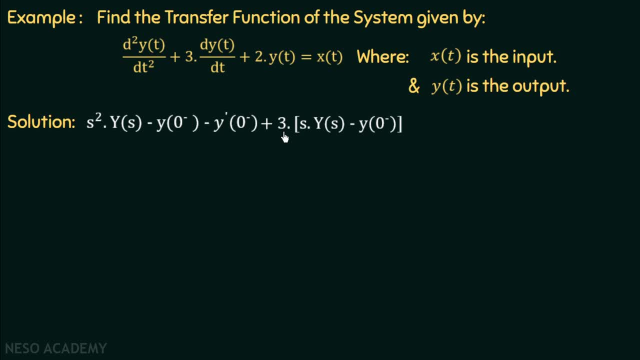 homogeneity. principle 3 will be multiplied in the Laplace transform. also. Similarly, the Laplace transform of 2 yt is 2 yt over dt. Similarly, the Laplace transform of 2 yt is 2 ys. And now the Laplace transform of xt is equal to xs And in this way we have: 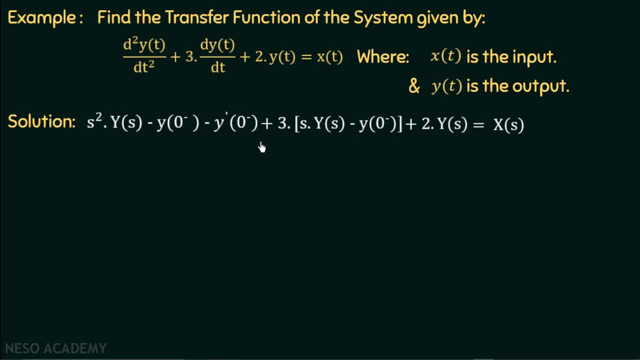 converted this differential equation to its Laplace domain And now we need to define the transfer function. But remember, to define the transfer function, the initial conditions of the system must be equal to 0. So the initial condition terms in this equation must be equal.